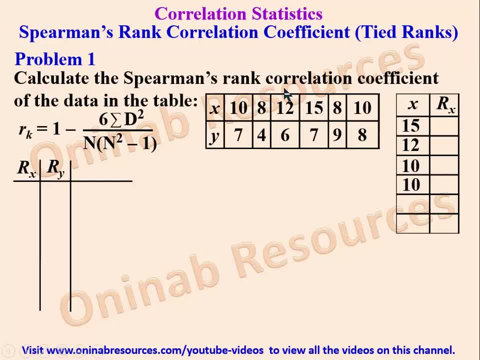 So we have 10 here, 10 here, 10 here been repeated and we have a 8, which is also repeated. then we now rank them. normally that will give us 1, 2, 3, 4, 5 and 6, so we now consider the ones that are. 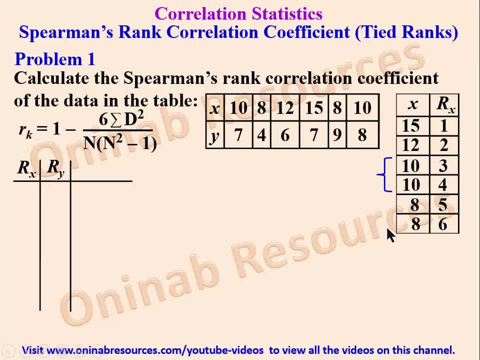 repeated. the 10 is repeated, 8 is repeated. so the ones that are repeated, we go to their ranks. we go to their ranks. that is for 10. the ranks are 3 and 4, so what we do is to find the average of this 3 and 4 and give it to them as 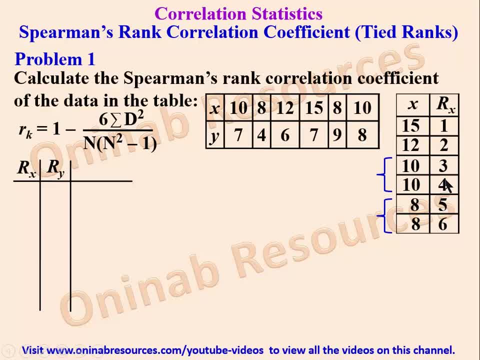 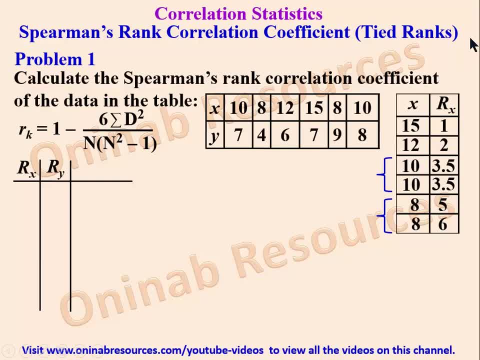 these 10s will be 3.5. so this is the method of resolving tied ranks in spearmint correlation coefficient. we now resolve the ranks for 8. the ranks are 5 and 6, so we add them divided by 2, that's finding the average 11 divided by 2. 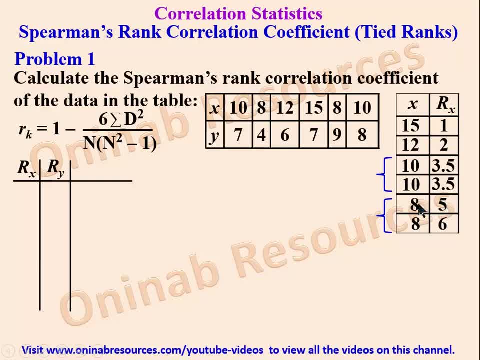 gives 5.5, so the new gives 5.5. so the new ranks for these two 8 will be 5.5, 5.5. so we now go ahead to assign the rounds: 200, so we have the versed value of X dare to be 10 and the. 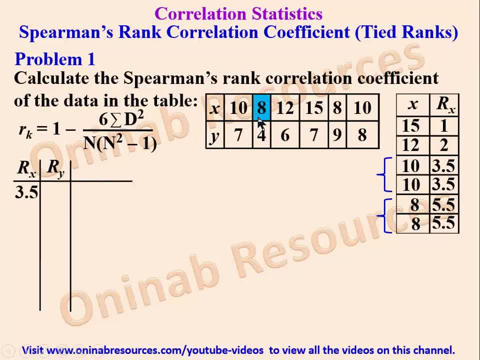 rank is 30 point five. the next value is 8, the rank is 5.5. the next value is 12堅 is 5.5, the next value is 12堅 12. the rank is 2, the next one is 15 and the rank is 1. we have a 8. the rank is 5.5, 10. 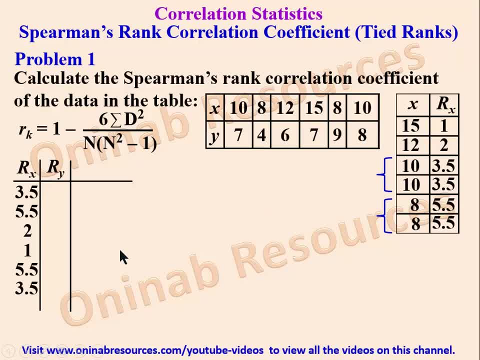 and the rank is 3.5. so we are done ranking X. so we now go ahead to rank Y. so again we arrange the values of Y in descending order. the highest value of Y here is 9. so we have 9, followed by 8, we have 7, and 7 is repeated, then 6, finally 4. we said 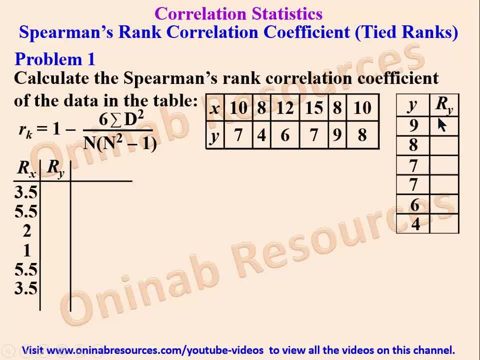 again. we rank them normally, so that will be 1, 2, 3, 4, 5 and 6. so we have 9, followed by 8. we have 7, and 7 is repeated, then 6, finally 4. we said 6, we now go ahead to consider the numbers that are repeated. then we resolve their ranks in this. 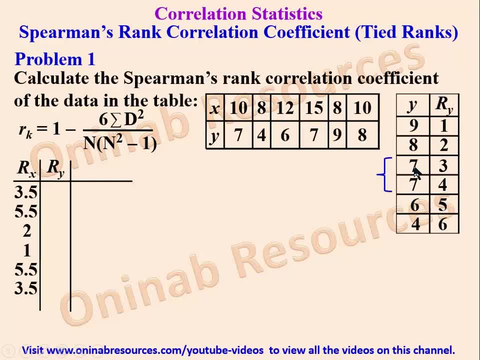 case we have 7 being repeated. so to resolve their ranks, we add this: 3 plus 4 gives a 7 divided by 2 gives 3.5. so their ranks now will now be 3.5. so 3.5 here, 3.5 here. 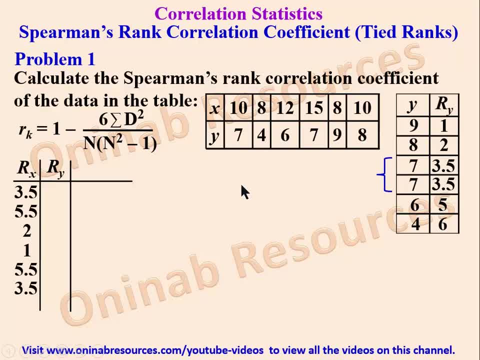 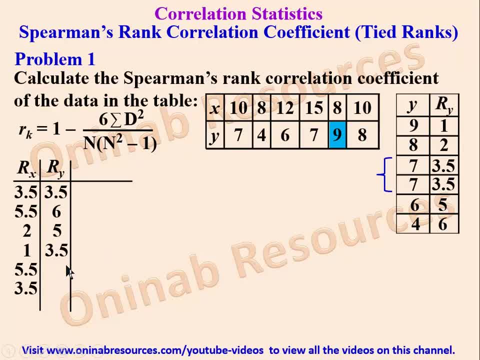 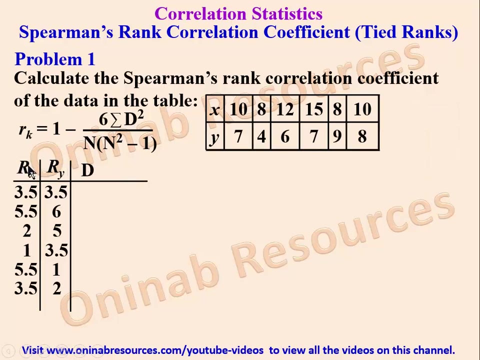 we have nine, nine, the rank is one, and finally we have eight and the rank of eight is two. so we are done finding the ranks of a, Y. so we now go ahead to find D, that is the difference between the ranks of X and Y. so we start 3.5 minus. 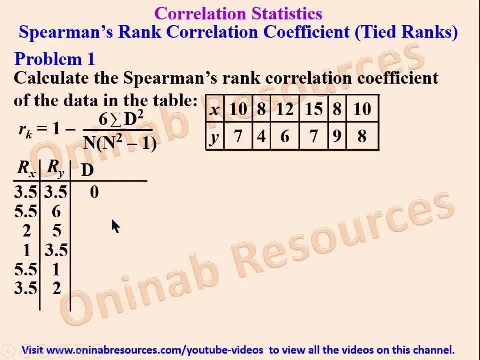 3.5 gives 0. 5.5 minus 6 gives negative 0.5. 2 minus 5 gives negative. 3. 1 minus 3.5 gives negative 2.5. 5.5 minus 1 gives 4.5. 3.5 minus 2 gives 1.5. then we find: 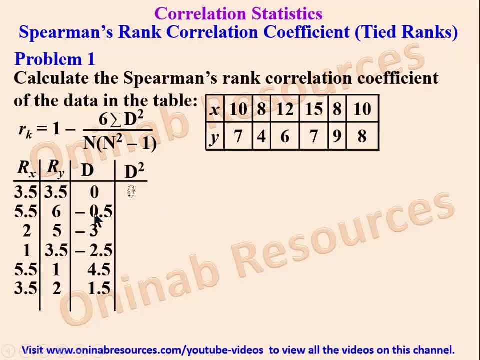 D squared, so square is 0. we have 0 square in negative. 0.5 gives 0.25. Squaring this will give us 9. Squaring 2.5 gives 6.25. Squaring 4.5 Gives 20.25. 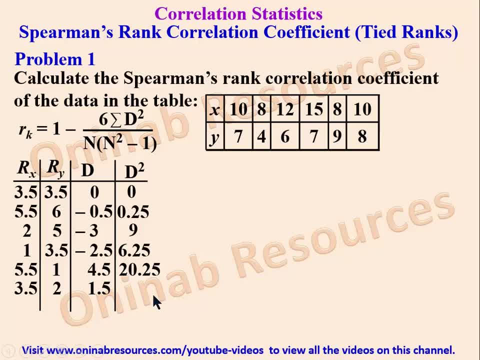 1.5 gives 2.25. So we are done. We now add this To give us the summation of d squared. So adding this, We can do that from our calculator. We have it as 38. So having gotten 38, We substitute into the. 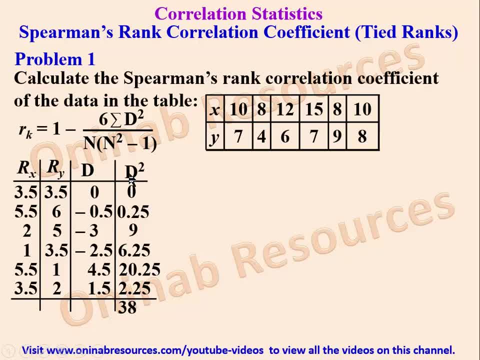 Formula for Spearman's Rank Correlation Coefficient, So that rk will be Equal to 1 Minus 6. Summation of d squared Is 38 Over The number of items we have here: 1,2,3,4,5,6. 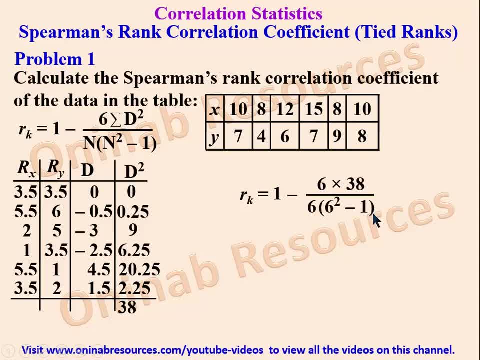 That's over 6 into 6 squared Minus 1. Here we can use calculator To resolve this. That will now give us 1.085714 And The final result gives Negative 0.085714, Which gives The Spearman's Rank Correlation. 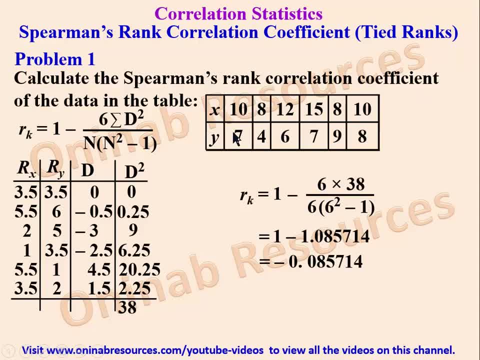 Coefficient Of the data we have In this table And the interpretation here is It is Negatively correlated. That is the interpretation. Remember we said The value of Spearman's Rank Correlation Coefficient Ranges from negative 1 To positive 1. So if it is close, 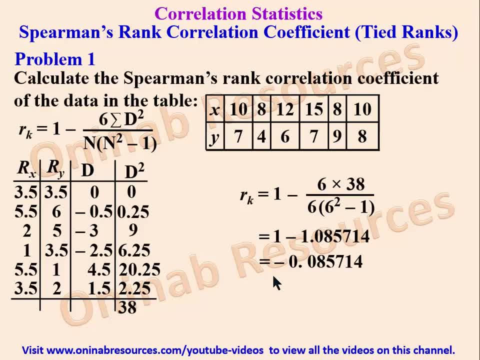 To negative 1, It is highly negatively Correlated. but if it is Close to positive 1, It is highly positively correlated. If it is very close to 0 From negative side, It is slowly negatively correlated, And if it is very close to 0 From the positive side. 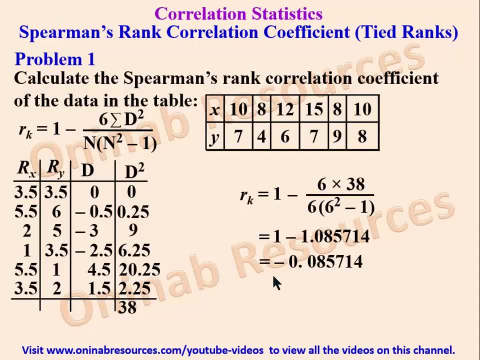 It is slowly positively correlated. So we can see this one now is It is close to 0 From the negative side. Not very close, Not very very close. So we still say Just negatively correlated, Though it is low. So we go to problem 2 For problem 2. 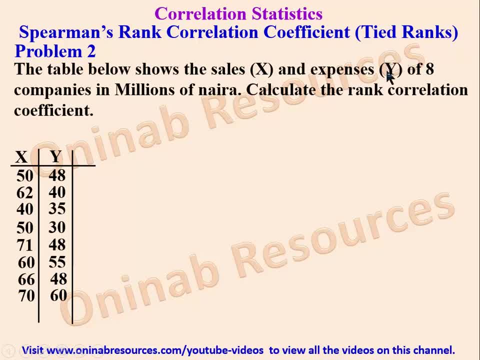 The table below shows the sales X and expenses Y Of 8 companies In millions of Naira, Calculate Rank Correlation Coefficient. So we are still talking about Spearman's Rank Correlation Coefficient. So we have our formula. Again, we are going to find the 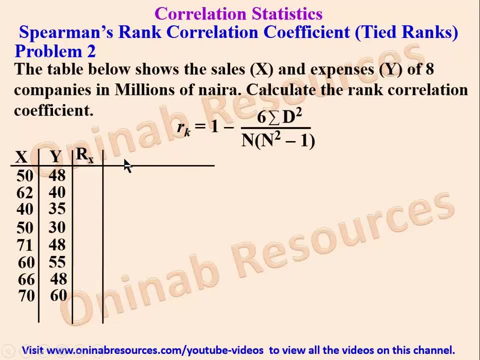 Ranks of X And the ranks of Y. To find the rank of X, We are going to rearrange X In descending order. The highest value of X there Is 71. So we have 71, Followed by 70, 66, 62, 60, 50. 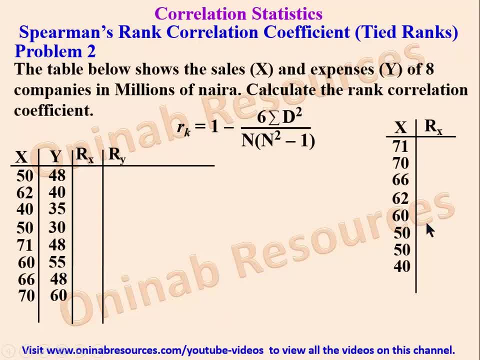 Is repeated twice, Then 40. We said we are going to rank them normally. That will give us 1, 2, 3, 4, 5, 6, 7 And 8. We now considered the repeated values And resolved their ranks. So the repeated values here are: 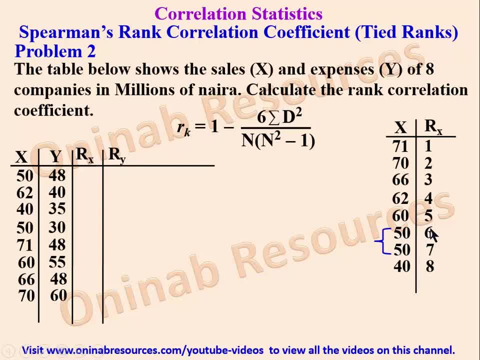 50 And 50. So to resolve their rank Is to find the average of their ranks. So that is 6 plus 7. Then divide by 2. Since there are 2 values, That will give us 6.5. So these 6 and 7. 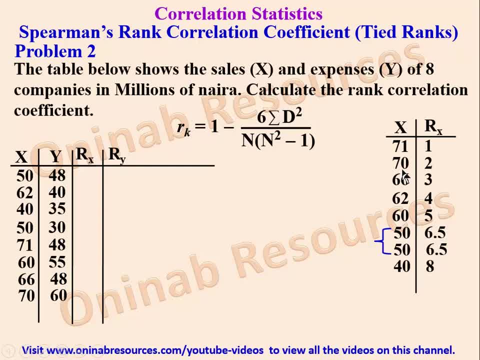 Will be replaced with 6.5 And we now assign each of the values Their ranks. For 50, We have 6.5 As its rank. 62 We have it as 4. 40 We have it as 8. 50 is 6.5. 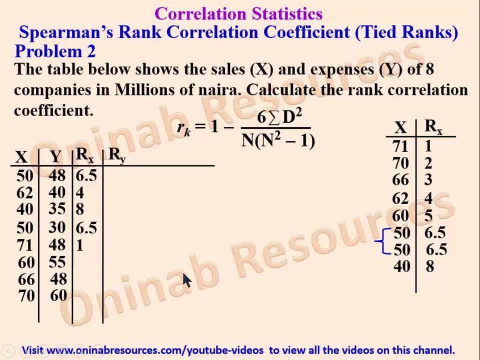 71, We have the rank as 1, 60 The rank is 5, 66 The rank is 3 And 70 The rank is 2. So we are done finding the ranks of X. We go ahead to find the rank of Y. So again, we arrange Y in descending order. 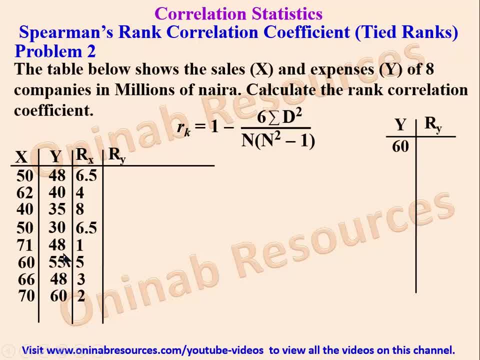 The highest value of Y, there is 60, Followed by 55. 55 is 1, 48, 48 is repeated thrice. So we have 48- 48 And we then have 40, 35 and 30. We said we are ranking them normally. 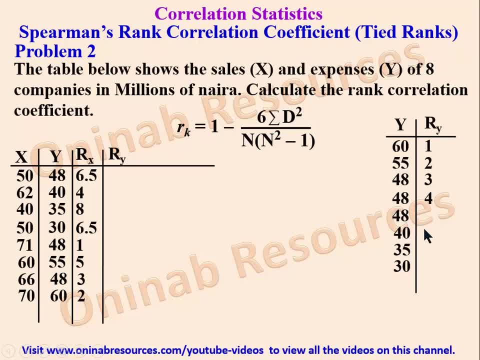 That is giving us 1, 3, 4, 5, 6, 7, 8. Then we now consider the repeated values, So that's 48. It's repeated thrice. We now consider their ranks. Their ranks are 3, 4 And 5, So we find the average of 3. 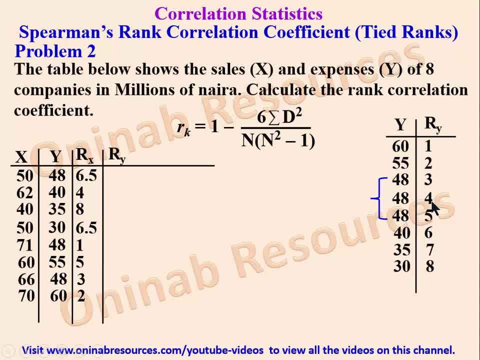 4 And 5. That will give us 3 plus 4. 7 plus 5, 5 gives 12. Then 12 divided by 3 Will give us a 4. So all these ranks now will be replaced with 4. Then we now go ahead to assign their ranks. 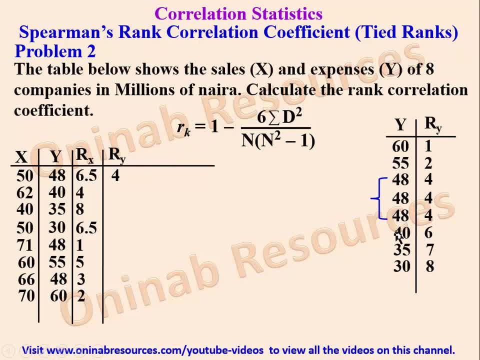 48. the rank is 4: 40. the rank is 6: 35. the rank is 7: 30. the rank is 8: 48. the rank is 4: 55. the rank is 2: 48. the rank is 4: 60. the rank is 1. 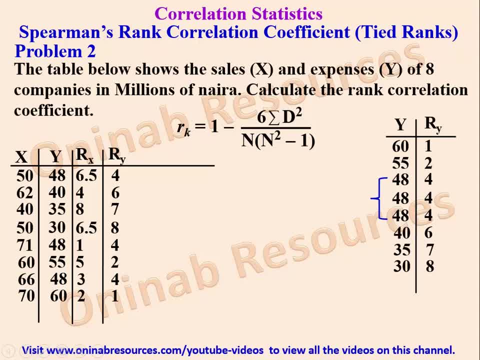 So we are done finding the rank of Y. So we now go ahead to find D. And then, D squared, 6.5 minus 4 gives 2.5. 8 minus 6 gives negative 2. 8 minus 7 gives 8 minus 7 gives 1. 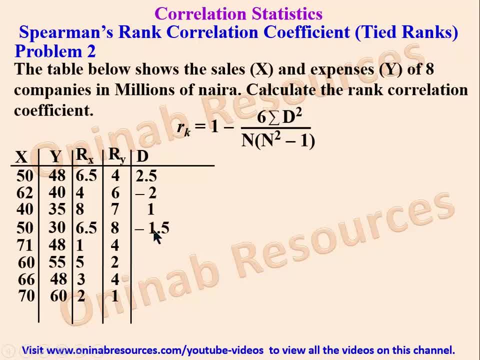 6.5 minus 8 gives negative. 1.5. 1 minus 4 gives negative 3. 5 minus 2 gives 3. 3 minus 4 gives negative 1. 2 minus 1 gives 1. So we go ahead to find D squared. 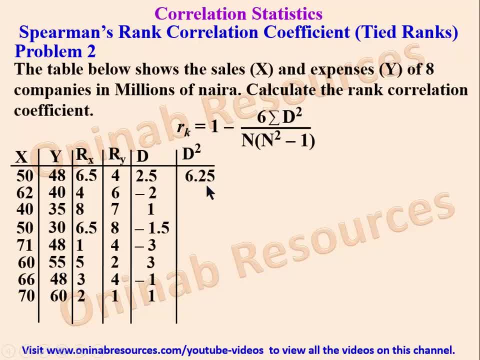 2.5 squared gives 6.25 Negative. 2 squared gives 4: 1, 2.5, 2.5, 1, 2.5, 1, 1 and 1 and 1. So, cameraman, give me a video. know what D is. 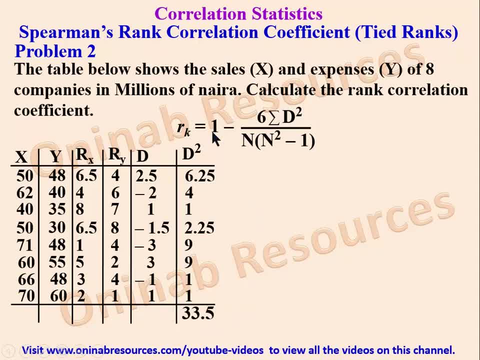 0.5, 0.5, 0.5, 0.5, 1, 1, 1, 2.25, 1, 2.55, 1 and 1, 2.25, 99, 1 and 1. point five over the number of frequencies we have here is eight into. 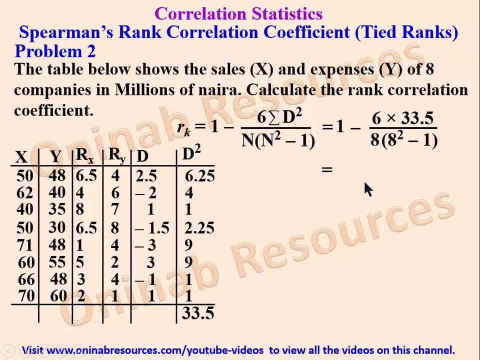 eight squared minus one, that will now give us one minus. evaluating this with our calculator, we have it as one minus zero point three, nine, eight, eight, so, and our final answer is zero point six, zero one, two. so the Spearman's rank correlation coefficient is positively correlated, and that is the end of. 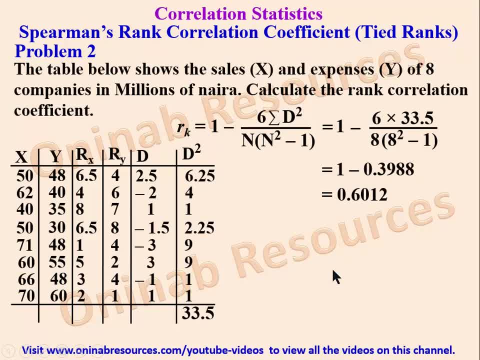 solution to problem two, and this is the end of this video. don't forget to check the description section of this video on our YouTube channel to get the first video on Spearman's rank correlation coefficient, without tied and ranks. until we come your way again, goodbye.